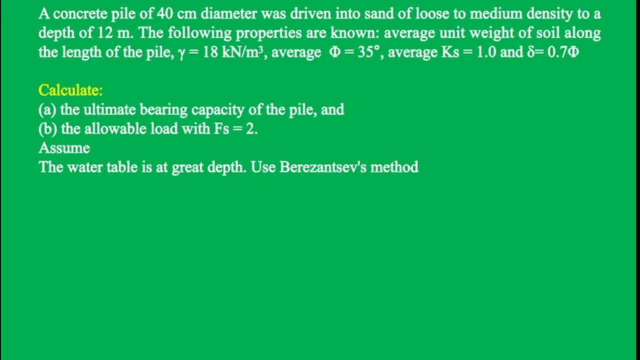 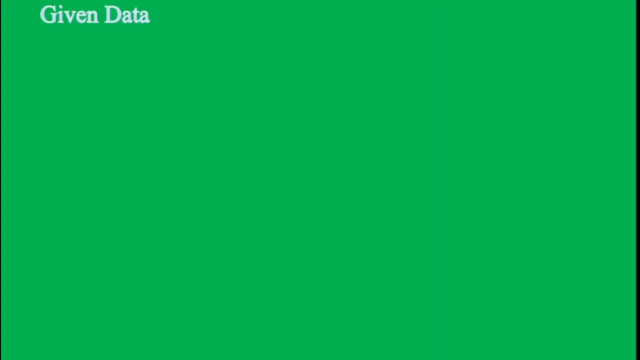 version saves method. this method we have seen in previous part. we'll apply this method in this video. Okay, so let's start. So, first of all, write down what is a given data. given data is this: pile is given and the pile has embedded depth of 12 meters. then we have: diameter is given 0.4 meter gamma. 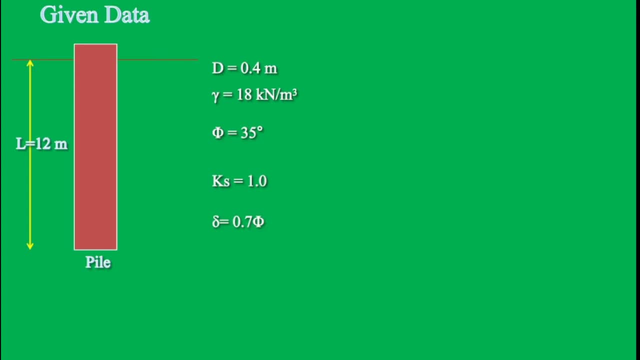 is given, Phi is given, KS is given, Delta is given, factor of safety is given 2. and now, next, we'll see how to solve this numerical. okay, so before solving any numerical, the best practice is to decide what will be your solution strategy. okay, here I have kept it very simple, so you already know. the formula for Q? u is: 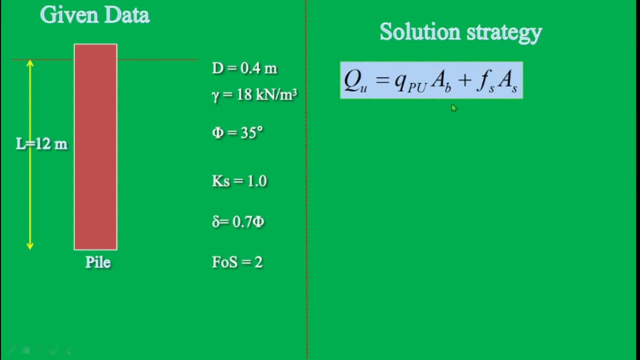 Q P U, that is, end bearing pressure multiplied by bearing area plus office multiplied by surface area. okay, so in step one we'll calculate all areas that are required, that is, the value of AB AS will calculate. in step two, we'll calculate the value of Q P U, so will calculate this. 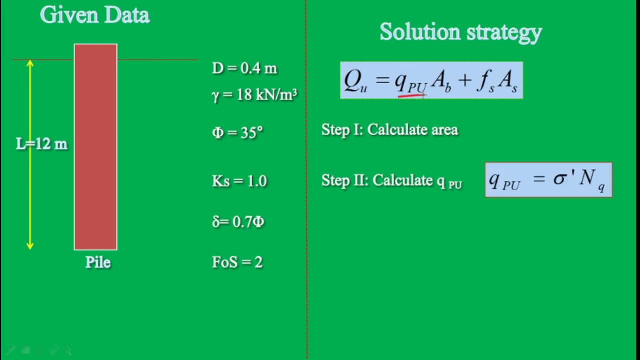 value as a last drink, helps me to estimate the value of Q P U, except one QPU, into the step 2 and in step 3. this is the formula for QPU- we'll see later on in detail and in step 3 we'll calculate the value of FS. okay, so once. 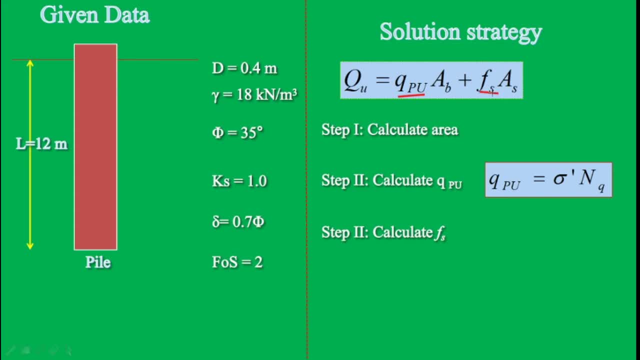 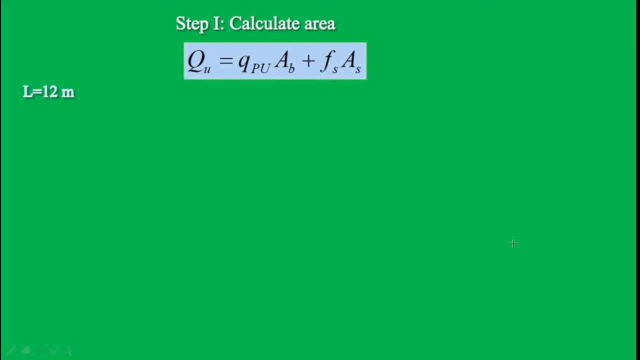 we do that, once we calculate the value of FS, we'll have all the values necessary for calculation of QU. okay, so that will be the formula for FS that we'll be using. so first step, calculation of area. so first area. so given properties are: length is given 12 meter, D is given 0.4, AB is a point bearing. 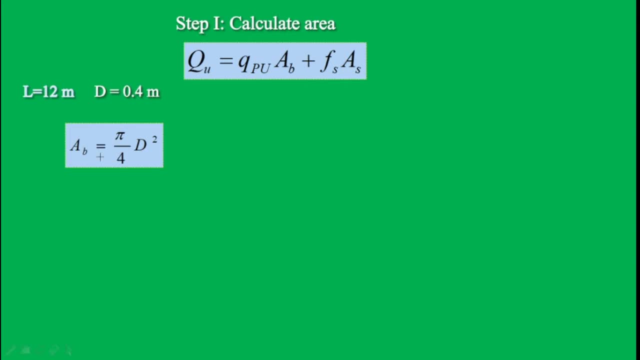 area. as it is circular, pile area will be pi by 4 into D. square D is given. so once you calculate that you will get the value of ABS 0.125 meters. square AS is nothing but the circular, sorry- surface area of the cylinder. so the formula is 2 pi rl, where r is a radius of the pile. that 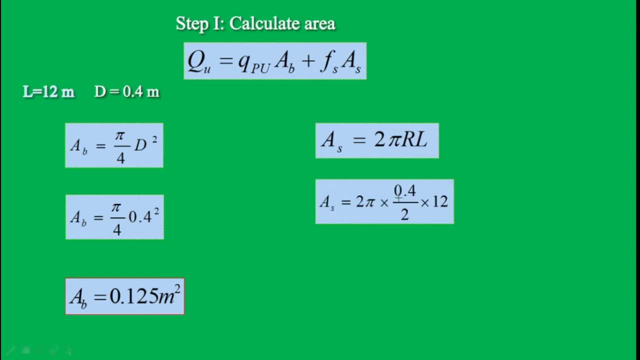 is t by 2, we have d is 0.4, so that value will become r, will become 0.4 by 2. once you put that value into the equation, you will get area as a 15.08 meter square. so we have completed our step. 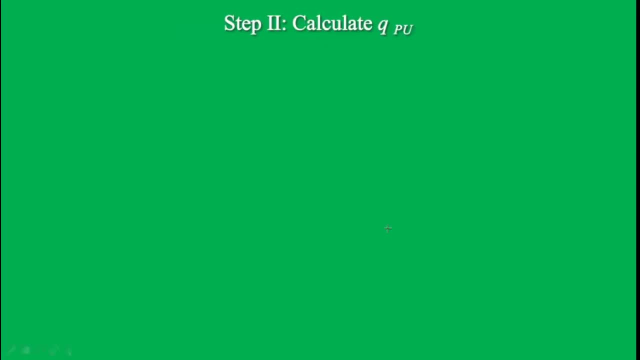 1. in step 2 we'll calculate the value of qpu. so in part 3 we have seen this is a formula for qpu, but as the given soil is a sandy soil, therefore c equals to 0. that means your value of qp in this. 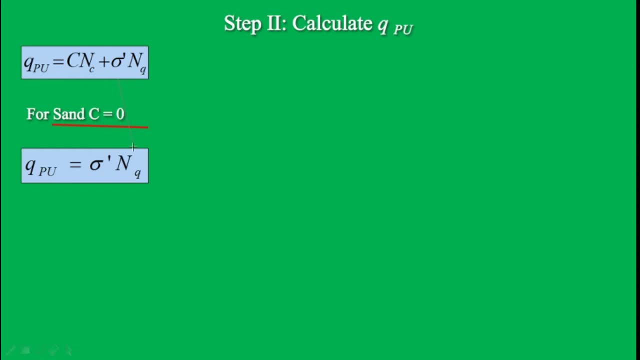 equation: once you put the c equals to 0, you will get qp, equals to sigma prime, into nq. okay, so next we'll calculate the value of nq. once you calculate the value of nq, we'll calculate the value of sigma prime. so let's focus on nq first. 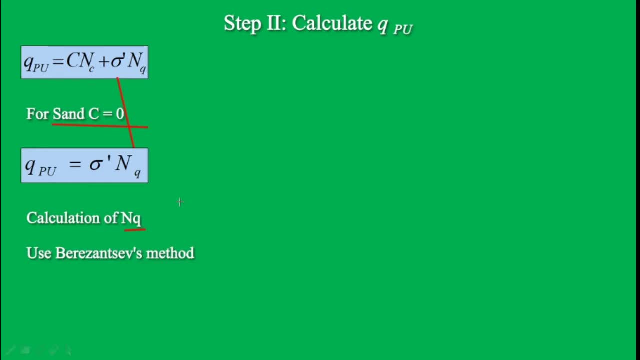 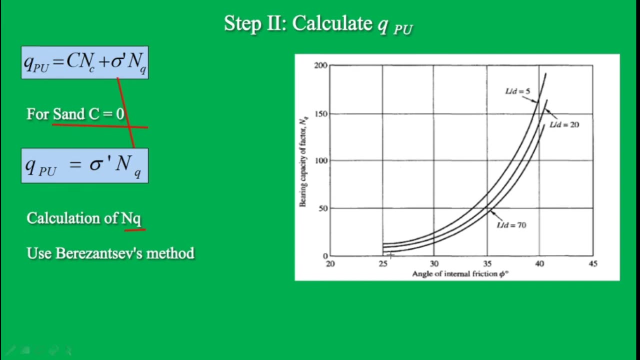 so we have to use berzantsev's method. what does this method gives? this method gives us this chart. by using this chart, you can calculate the value of nq. so what are the factors that are required? first thing, we need the value of angle of internal friction, that is, phi. phi is given to us 35. 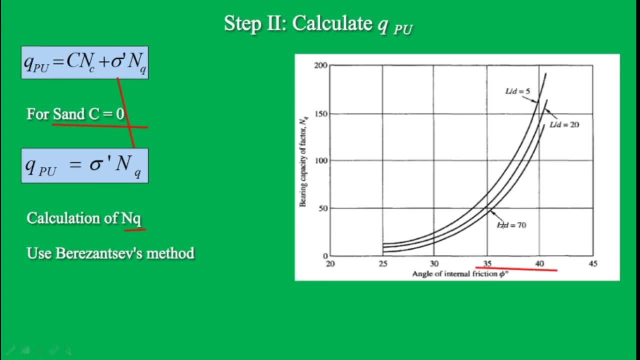 angle of internal friction. that is, phi phi is given to us 35. that is, phi phi is given to us 35, no need to worry about it. next, we need l by d ratio. so for our soil, so for our numerical, l is given to l, d is given 0.4. so your l by d ratio is 30 and your phi is 35. so let's go to this 35. 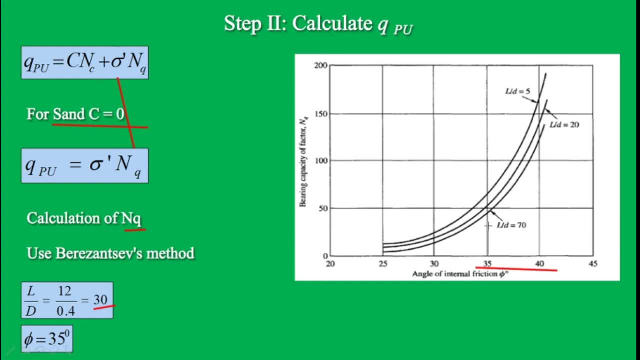 and l by d. this 30 will be somewhere over here, so from this you can calculate the value of nq will be just a little bit below 50, so that value i have taken as 48, so nq will be 48. this is how we'll use berzantsev's method to calculate the value of nq. there is a one more method. 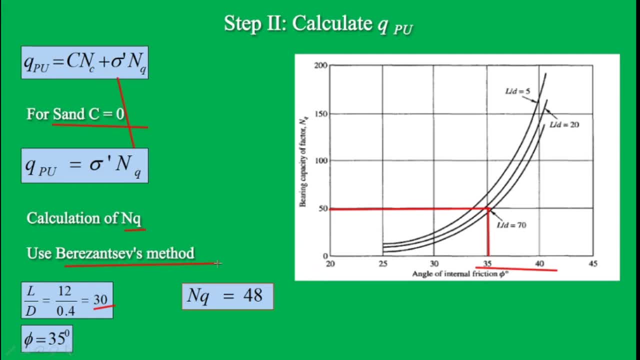 given by the mayerhoff. you can also use that method, but the numerical is specifically mentioned to use this method. so we have used berzantsev's method. okay, so in the value of nq we have to use value of qpu. if you have calculate the value of nq, our next task will be calculate the value of. 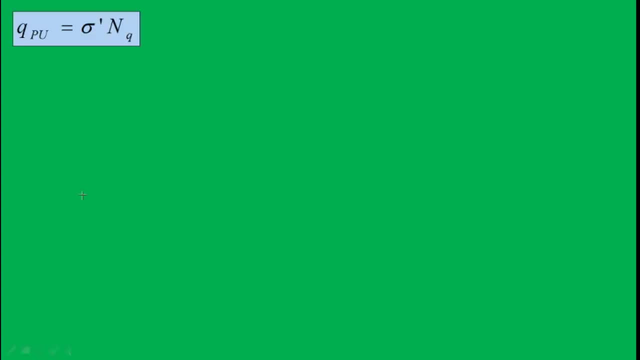 sigma prime. so sigma prime equals to gamma- into lc. this is again we have seen in our previous video. now this lc gamma, sorry sigma is given to us, sorry gamma is given to us, 18 kilometer per meter. q will not have to worry about it, but the value of lc we have to calculate. this lc is nothing but. 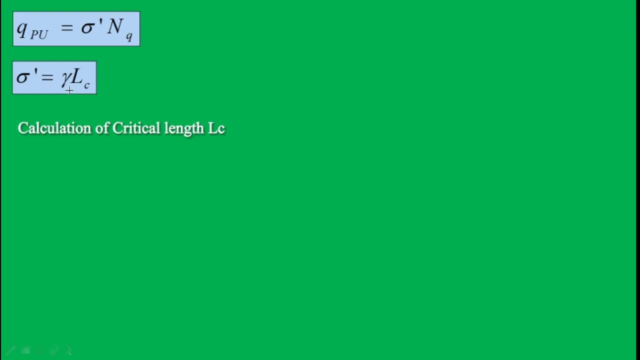 critical depth of the critical length of the pile. so, as we have seen earlier, critical length of the pile for loose to medium sand is 15 times of d. so we have value of d. lc equals to 15 times of d, our d is 0.4, l is, so your lc becomes 15 into 0.4. that is 6 meter. so you have got the value of. 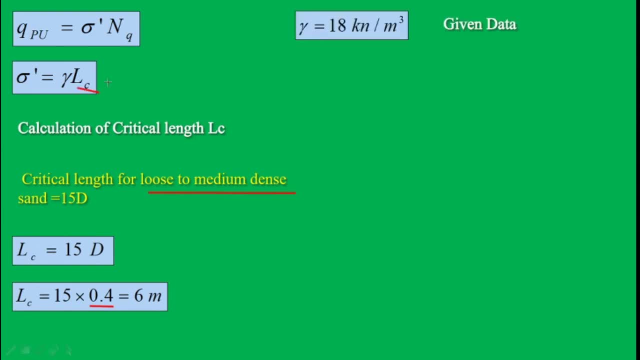 lc over here so you can easily calculate sigma prime. sigma prime is equals to this gamma. that is, 18 multiplied by 6, you will get the value of sigma prime as a 108 kilometer per meter square. as it is stress, its unit will be kilometer per. 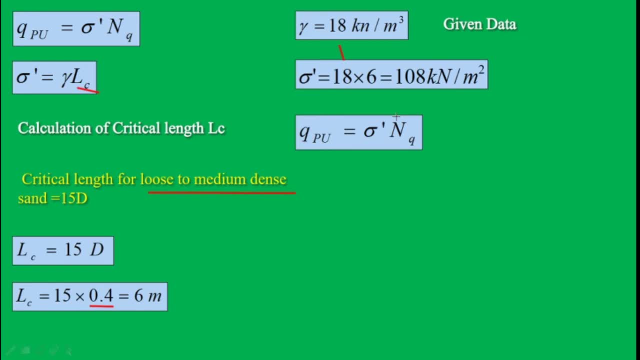 meter square. next, so for to calculate the value of qpu. we have both nq. we have calculated using berzantsev's method, sigma prime, we have just calculated. so your value of qp equals to 5184 kilometer per meter square. so this is how we reach to our step number two. okay, so till this. 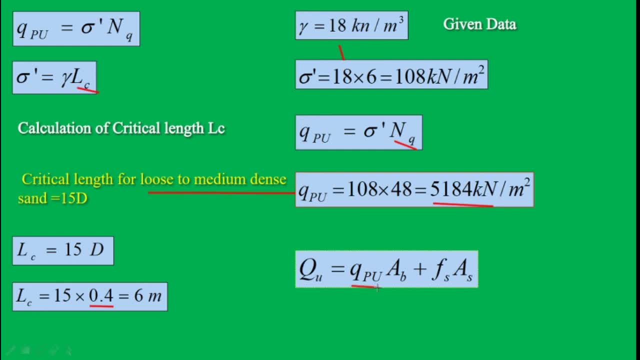 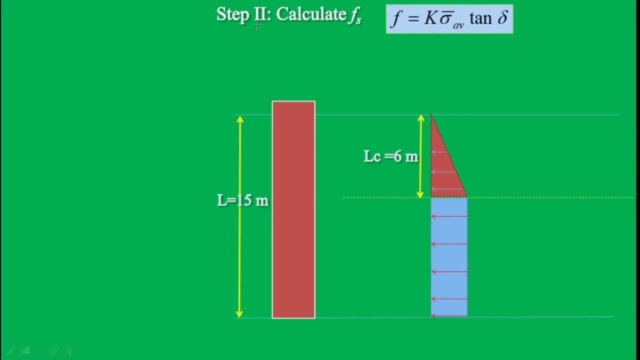 step what we have calculated. if you have calculated qpu, we have calculated ab, we have calculated, as the only thing remaining is calculation of fs. that is our step number three. actually, this should be step number three, not two. please correct it. so the formula for fs is: 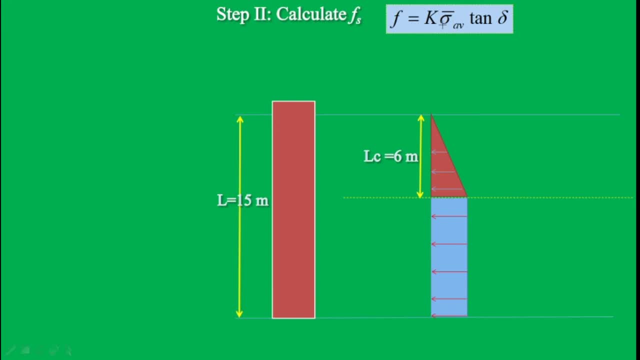 very simple k into sigma average multiplied by tan delta. so, as you can see over here in this- we have also seen this in previous part- there are because of this critical length lc, we have two parts of stress variation. the part one is from 0.0 to lc. your stress increases in a downward direction. 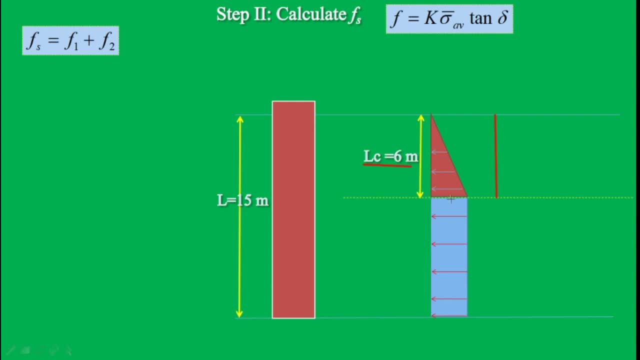 but it only increases up to the value of lc and after that your stress remains constant. okay, so basically you have two different type of stress distribution. so your fs will be addition of f in this area for this diagram and f in in this area. okay, so we'll calculate, we'll add. 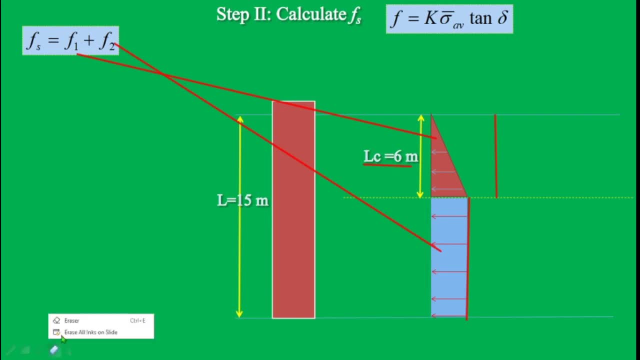 stress variation in both of these areas and we'll get the value of fs. so first, to calculate the value of fs, we need sigma av. to calculate the value of sigma av, we need the value of sigma at this level. at this level, the value of sigma will be very simple, or gamma into lc. 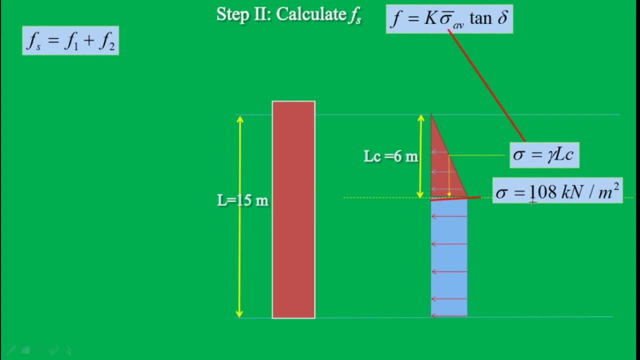 gamma into lc. we already seen that value comes as a 108 kilonewton per meter square. so at this level let me rub it out. this is a very important step. if you don't understand anything, please comment down to the video. i'll explain you one more time. okay, so at this level you've got. 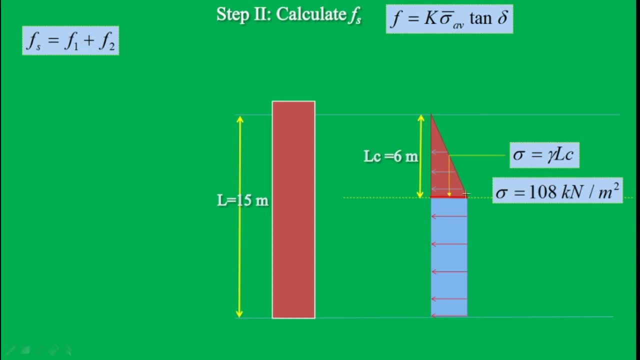 sigma as a 108 and after that that sigma 108 is constant till the bottom. okay, so that's why, at the bottom again, you will get the value of sigma as a 108. now how do we calculate the value of sigma av1? what is this sigma av? because this f1 will be equals to 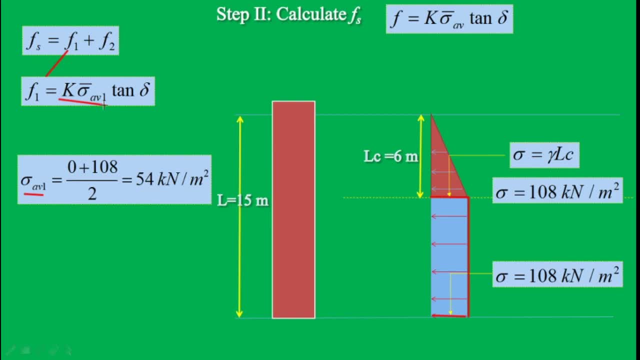 j sigma av1 into tan delta. this sigma av1 is related with this triangle. so this sigma av1 equals to average. this av stand for average, for diagram number one, that is, triangle. so how do we take the average? average will be equals to 0 plus 108, so 0 at this point at the top, 108 at the bottom. 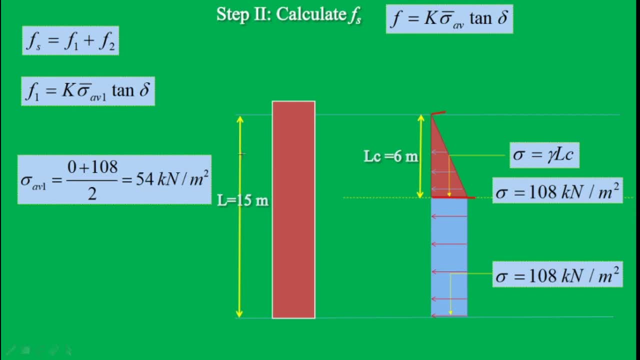 okay. so 0 plus 108 divided by 2 will give you 54 kilo newton per meter square. that is sigma average for the. this figure triangular one. okay. similarly, sigma av2 is related with this figure. now, in this figure there is no zero value at the top, it is 108 at the bottom. 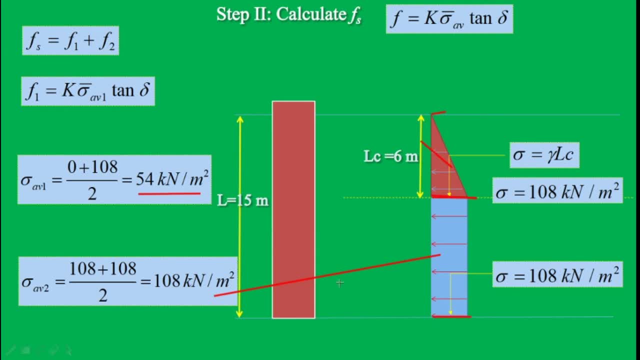 again, it is 108. so average will be equals to 108 plus 108 divided by 2, that is 108 kilo newton per meter square. so in order to calculate the value of f1, you need sigma av1 and sigma av2, which we have just calculated. so what we'll do, we'll calculate. 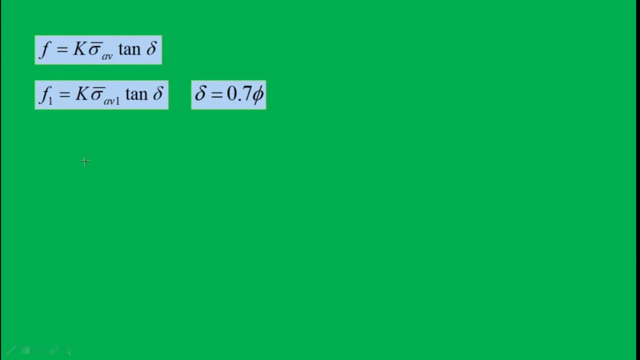 the f1, then we'll calculate the value of f2. then we'll add f1 plus f2, we'll get the value of fs. so f1 equals to. the formula is here: k is given 1 sigma, av1, 54. we have just calculated tan delta and. 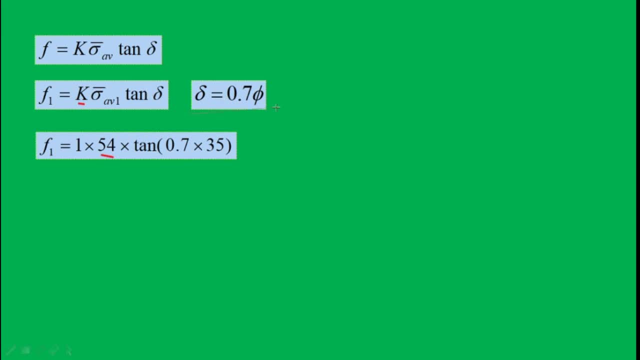 delta is nothing but 0.7 times of phi. phi is 35, which we have put over here. so your value of f1 equals to 24.60 kilo Newton per meter square. similarly, we'll calculate the f2. this is your k, this is your sigma av2 and this is your tan delta. so your f2 equals to 49.21 kilo Newton per meter. 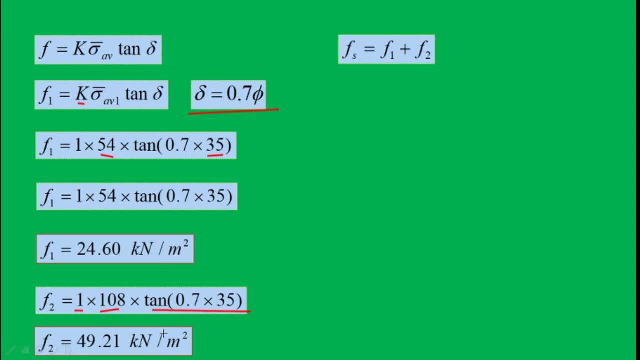 square. okay, so the only thing remaining is calculation of f1.. of fs, that is f1 plus f2. just add these values to this value we have calculated over here. f2- we have calculated over here. add these two value, you will get the value of fs as 73.81 kilometer. 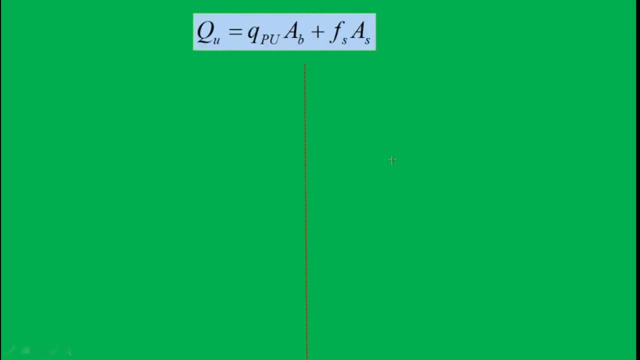 per meter square. so, for our final formula qu, what we needed, we needed all these values which we have just calculated over here. i have given it for your reference. you should check all the calculations, okay, so once you put these values into this equation, you will get this. 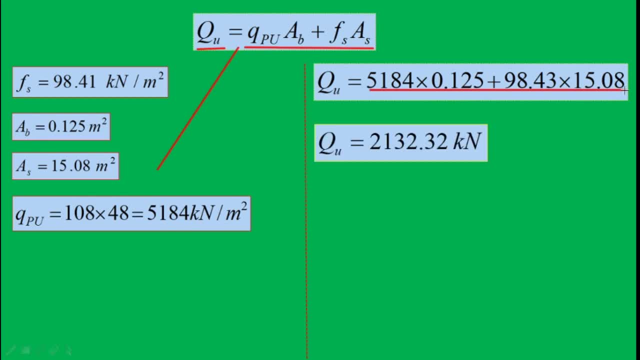 equation, just solid. just calculate it. you will get the value of qu as 2132.32 kilonewton. that is nothing but your ultimate load carrying capacity, that is, ultimate pile load. this is the first thing that we have been asked to calculate. second thing: we have been asked to calculate the 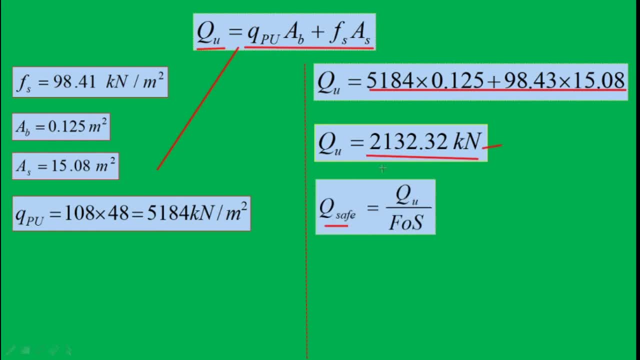 value of q safe. q safe is nothing but this. qu you divide by factor of safety, factor of safety is given two. so once you divide this value by two, you will get the value of q safe as a 1066 kilonewton. okay, so this is how we solve the.